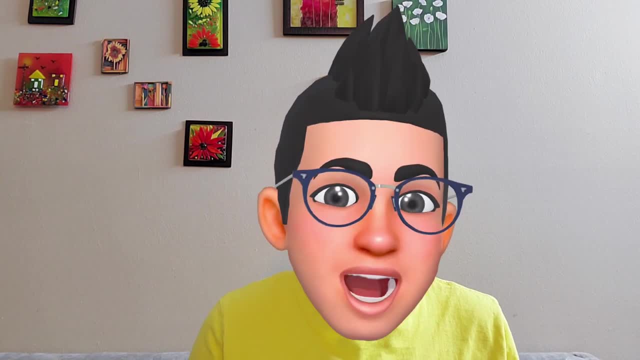 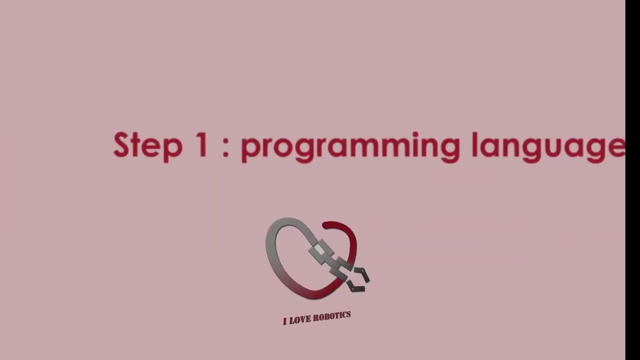 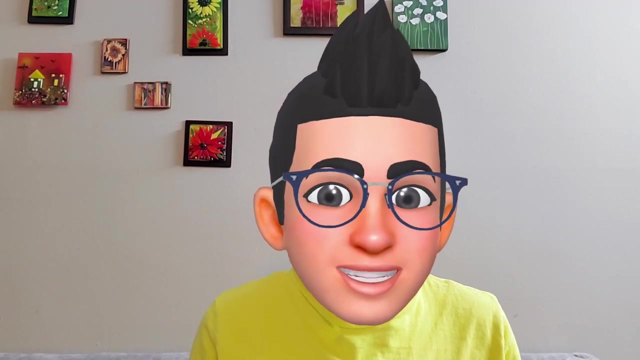 to be able to build a robot car and program it. if you are an absolute beginner with no prior knowledge of programming or electronics, Let's get right into it. Step number one: programming language. The first thing you need to learn is a programming language. Now you may ask: why do I need to learn a programming language, Dr Robot? 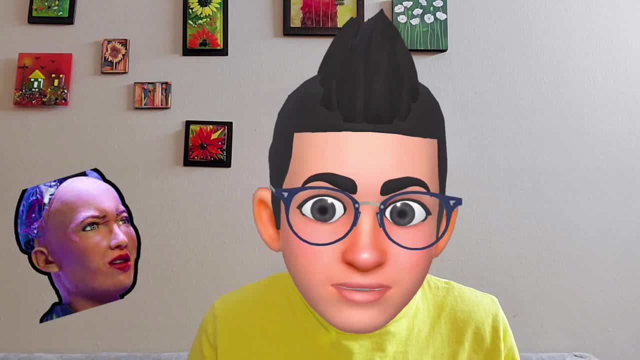 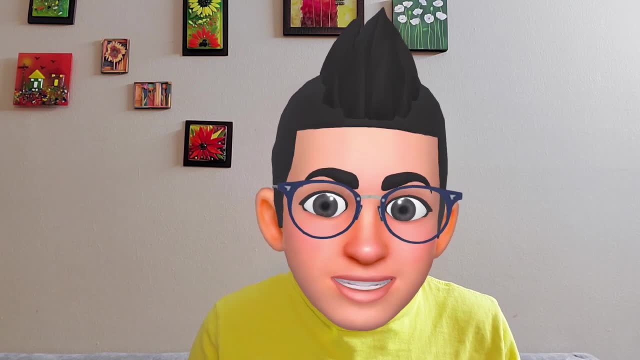 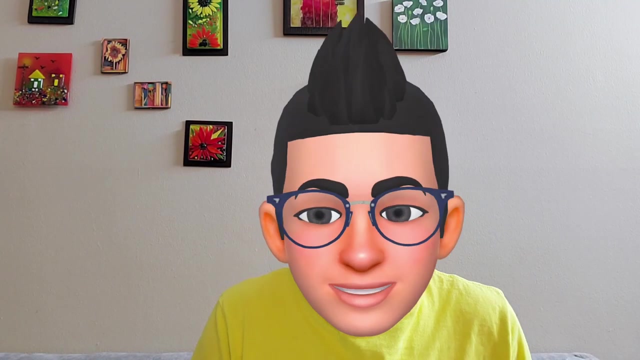 Well, the real reason is, robots are dumb. before they are programmed, You need to tell them exactly what they need to do, step by step. These precise, step-by-step instructions are communicated to the robot via a programming language. Okay, Dr Robot, I agree I need to learn a programming language, But 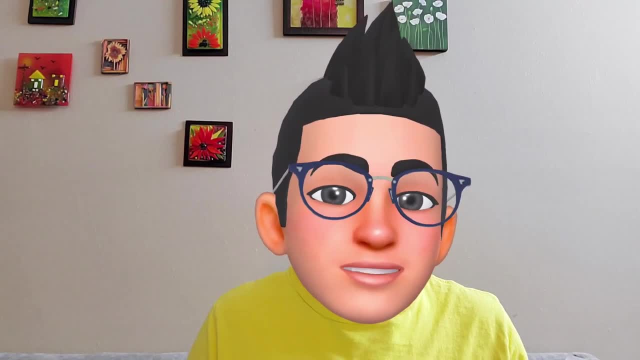 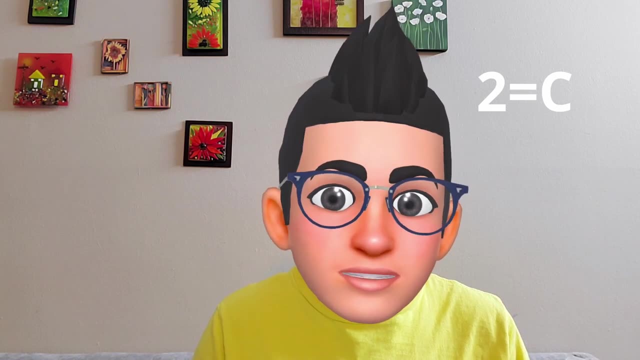 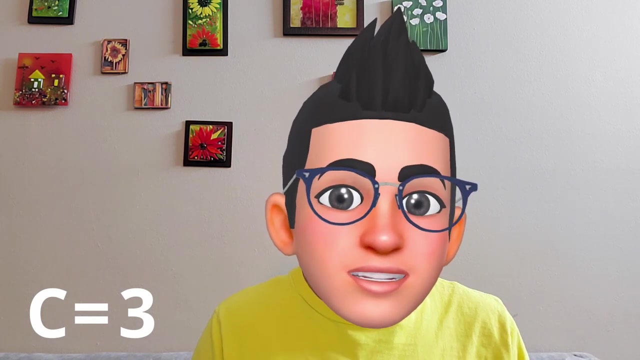 what programming language do I need to learn? I'm glad you asked. As a beginner, the best programming language for you to learn is C. C is the language used to talk to electronics and hardware. C is also used to program an Arduino board, which we will talk about next in this video. Also, C is a pre-req to learn C++. 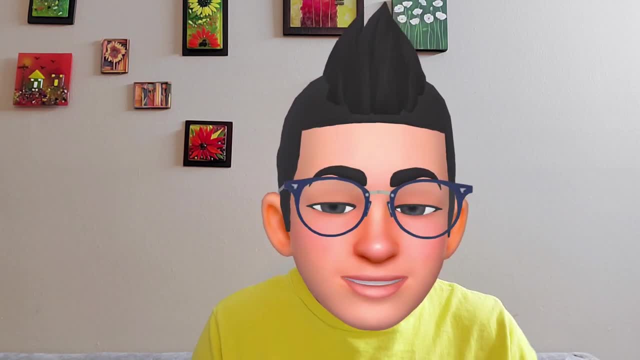 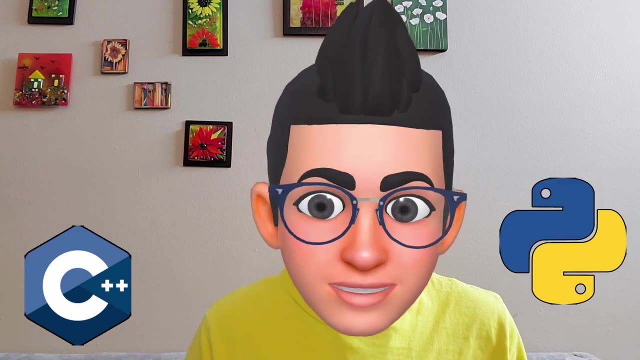 which is the most used programming language in robotics? Oh wait, Dr Robot, I'm confused. now Do I need to learn C++ as well? And then how about Python or Java? No worries, I understand why you are confused, But, lucky for you, I have created a video that 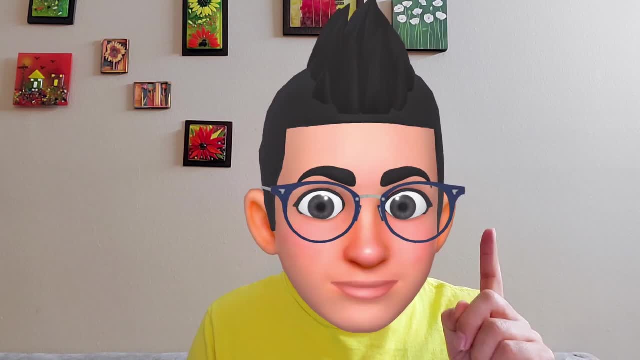 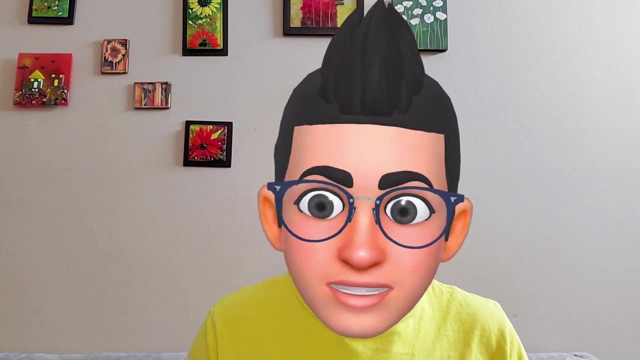 answers that question. Please refer to the card above or the link down below in the description, so you don't miss it. If you want to learn more about C++, go to the link in the description. But again, as a beginner and to start, just learn C. 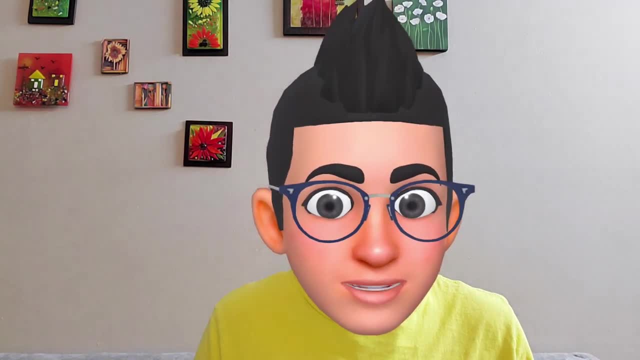 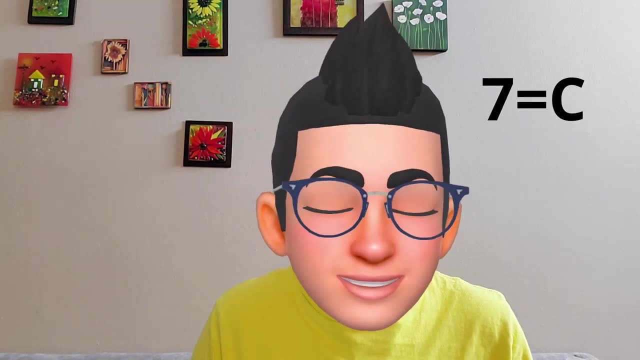 Thank you, Dr Robot. Now I know what a programming language is and I know, as a beginner, I need to learn C. But is there any online course I can take to learn C programming? Sure, there is. I have done my research and here is one of the best online courses to learn C for. 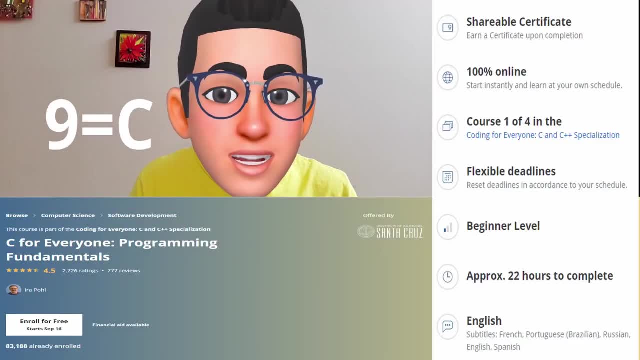 beginners. This course is called C for Everyone and it's offered by University of California Santa Cruz, and it's available in English, Spanish and Spanish, And it's on Coursera platform. The course will teach you only the basics of C. 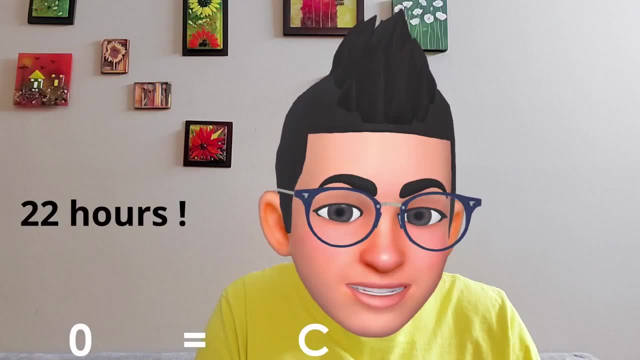 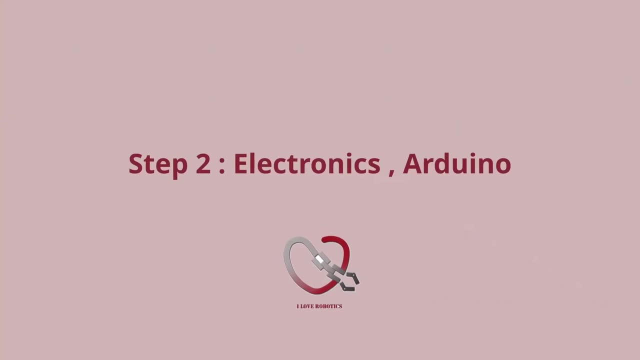 and it should not take you more than 22 hours to complete, which means if you spend 3-4 hours a day, you should be able to complete the course in less than a week. Step number two: electronics. Now that you know C programming language. 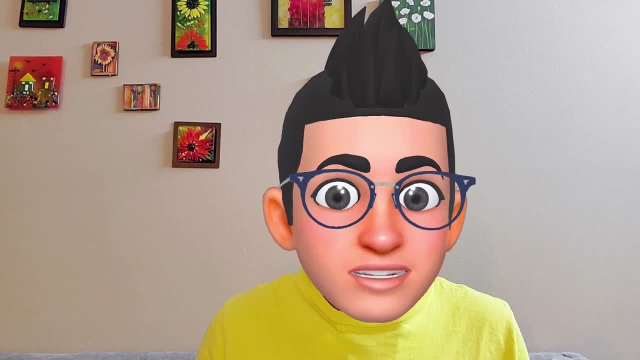 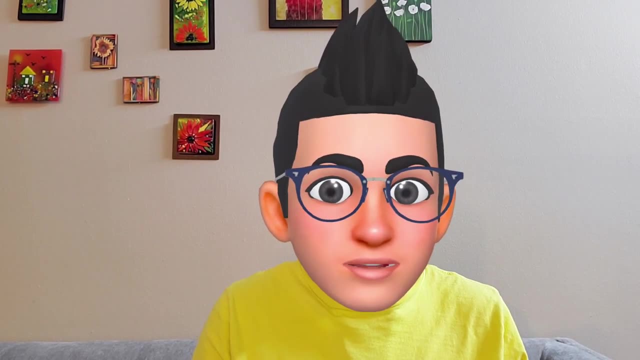 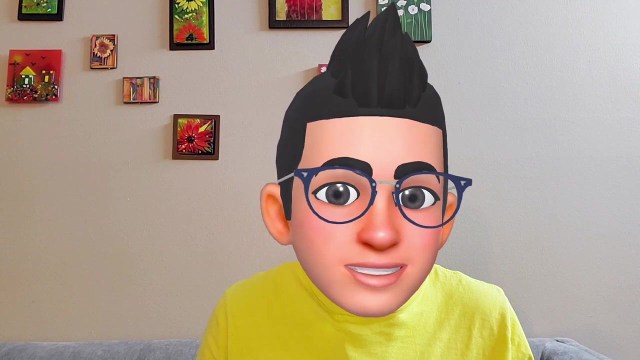 it's time to learn electronics. You can learn electronics using an Arduino board. But what the heck is an Arduino board? Arduino is an easy-to-use controller board designed for beginners with no prior knowledge of electronics to do cool projects, Projects like atomic clock, drones, 3D printers, robot cars and many more. 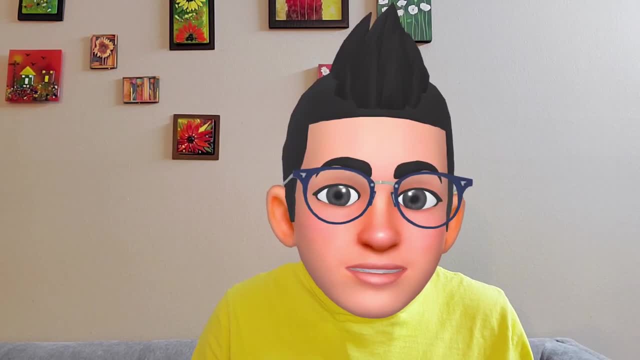 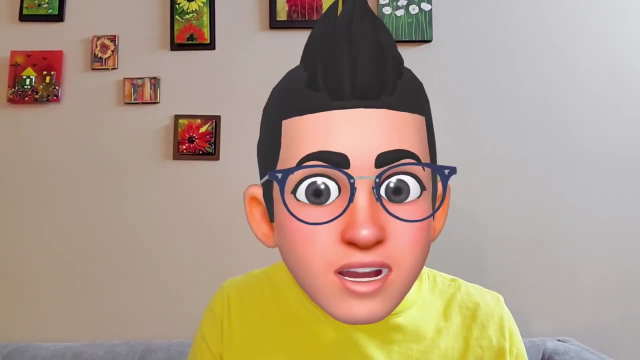 Arduino is essentially a small computer that you can use to receive inputs from sensors and command actuators, such as electric motors, to do stuff. Arduino is programmed in C. Now you know why you need to learn C right. And then it comes with its 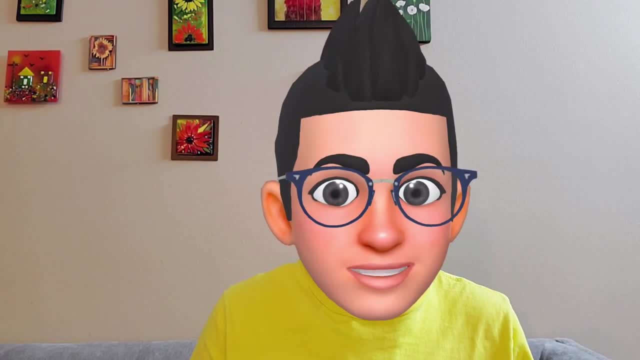 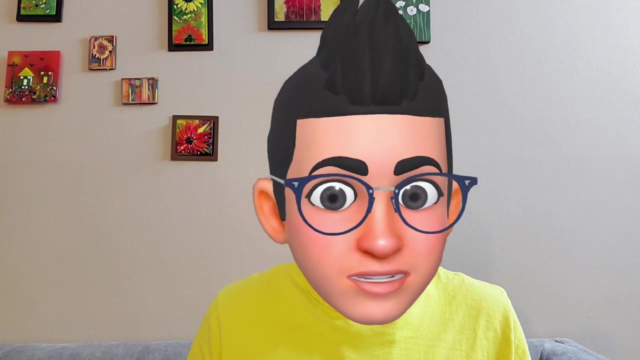 hardware. Arduino is very popular among hobbyists and makers. Arduino is even used in the industry. I still use Arduino. It's used to rapid prototype ideas and to build test fixtures. So, first thing first, you need to buy an Arduino board, right? So I'd suggest you buy an Arduino. 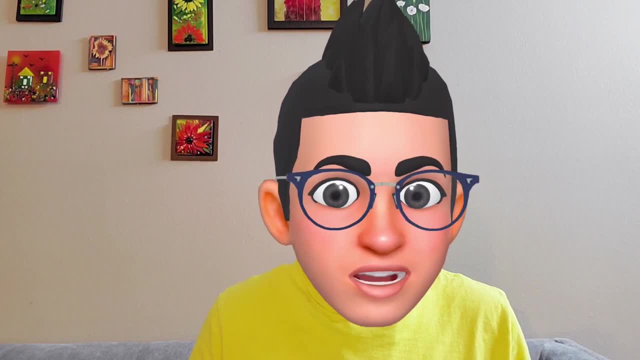 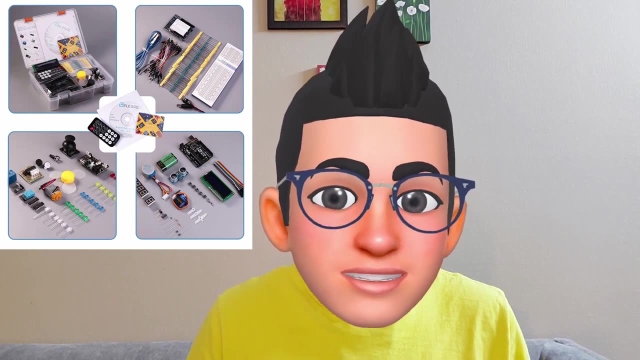 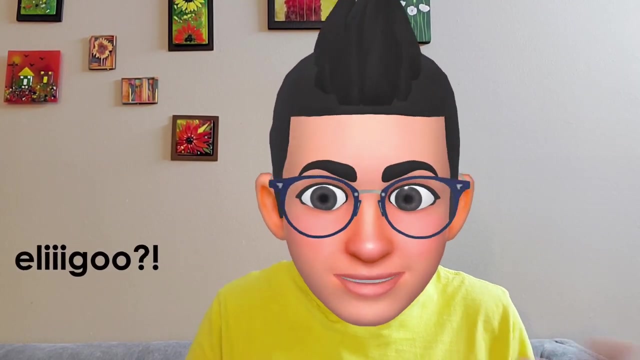 kit that comes with the Arduino board and all the other electronics, such as sensors, wires, jacks and motors. So I've done some research and I found this Arduino starter kit by Elegoo- Is that how they say it? Elegoo, Elegoo, I don't know Whatever that is. 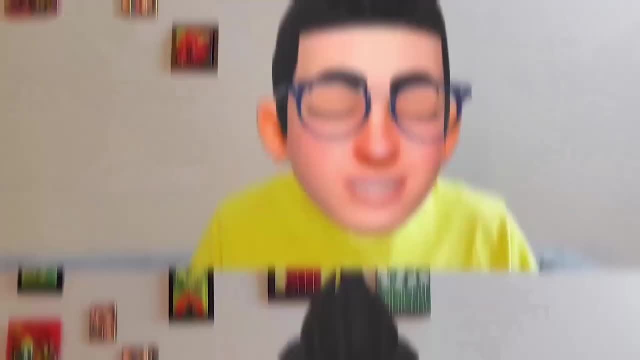 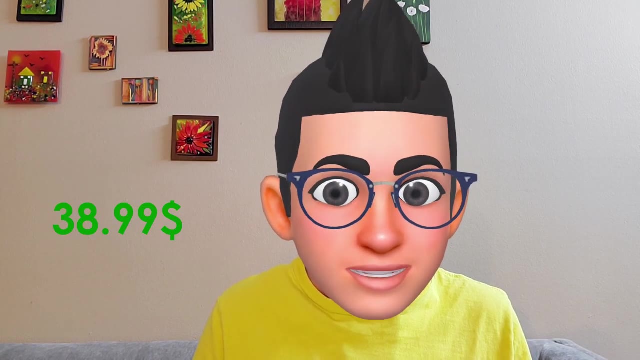 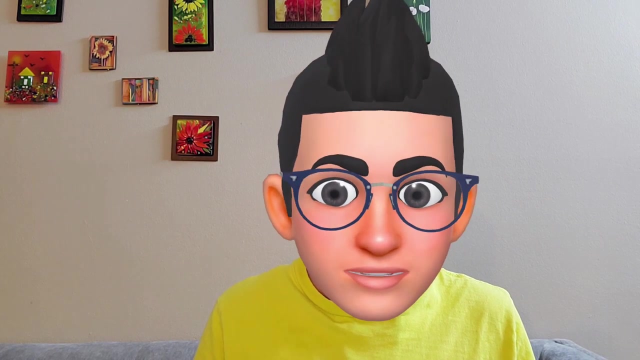 you can find it on Amazon. The link would be down in the description section. So this Arduino starter kit by Elegoo is a great and complete kit to buy. It runs for $38.99 on Amazon And I've contacted Elegoo and they've been nice enough to offer some promo code for additional discounts. 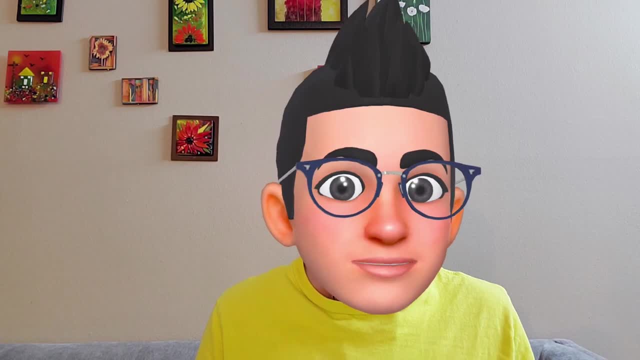 So the discount and the link will be down in the description section. Please note that this video is not sponsored by Elegoo. If you're interested in learning more about Arduino, please click on the link in the description section. And if you're interested in learning more about Arduino, 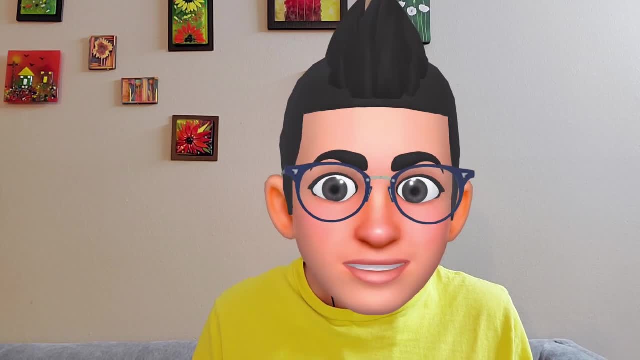 please click on the link in the description section. And if you're interested in learning more about Elegoo, please click on the link in the description section. And this is just just my personal opinion on a kit that you can find on Amazon. The Elegoo Arduino kit is loaded with sensors. 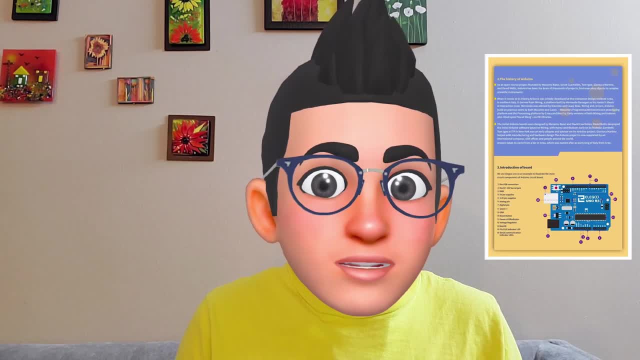 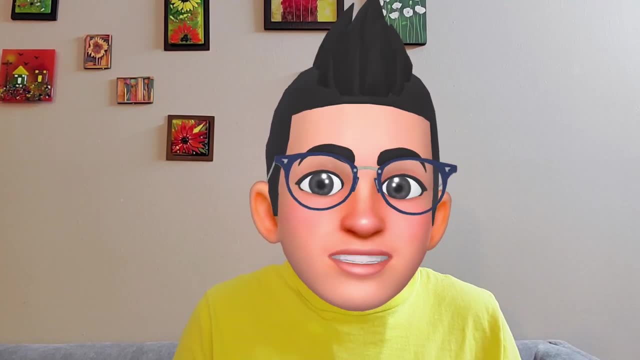 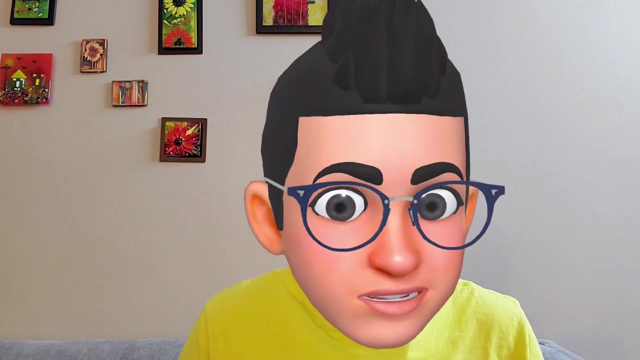 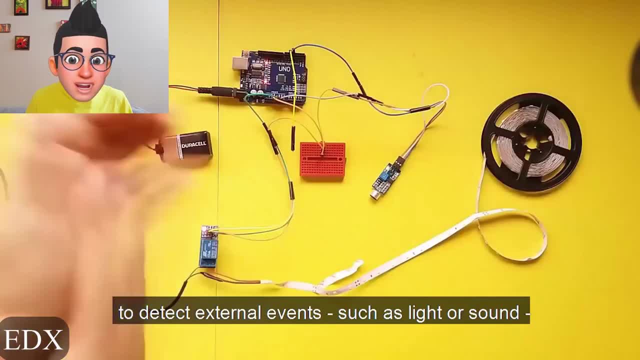 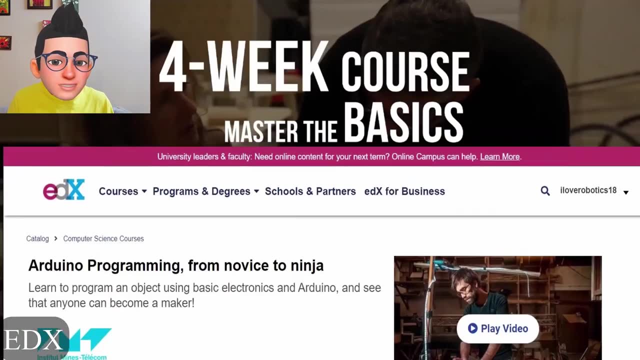 take this course on edX to learn how to do some cool hands-on projects with Arduino. You should be able to complete this course and learn how to use Arduino in less than three weeks if you spend three to four hours a day, or maybe just a week if you put in enough time each day If you live in. 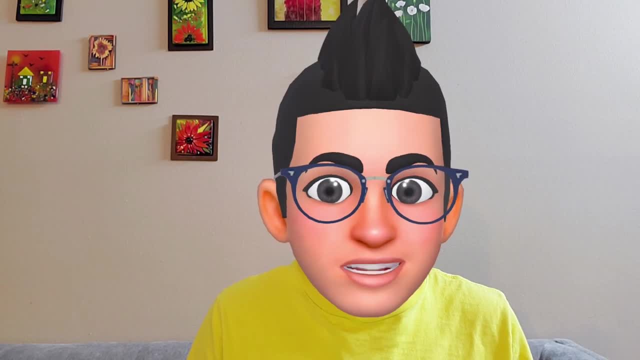 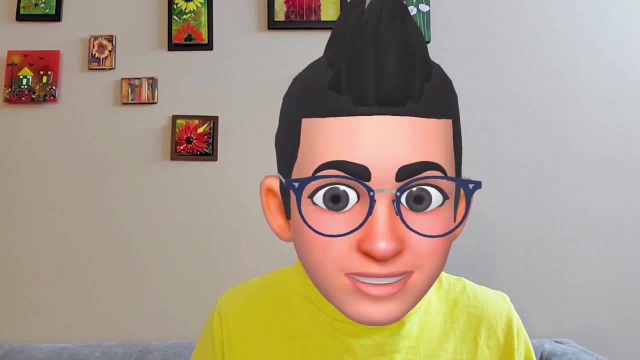 a country that Amazon does not ship to. please refer to the description section for additional resources. Also, comment or contact us, and we'll do our best to help you get an Arduino kit. Now you may ask: can I use Raspberry Pi instead of Arduino? The short answer is yes. However. 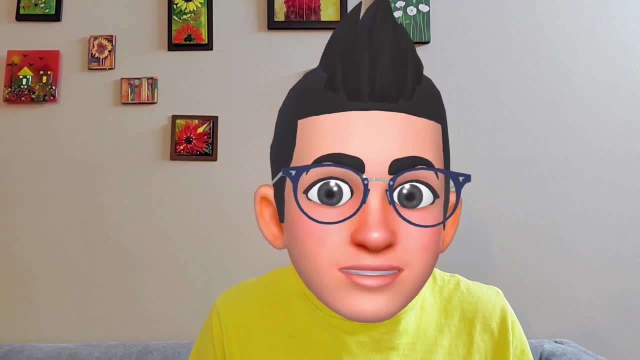 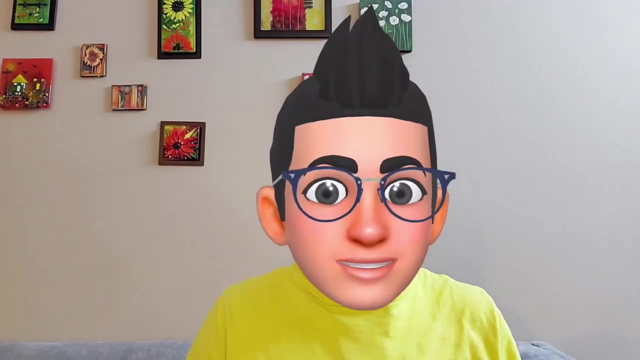 again, as a beginner, it's better to start with Arduino, because Arduino is much easier to learn, has more training resources and is much more popular. Step number three, and the most exciting step, is build and program a robot. All right, In step one, you learn C. In step two, you learn how to use C to program an Arduino board. 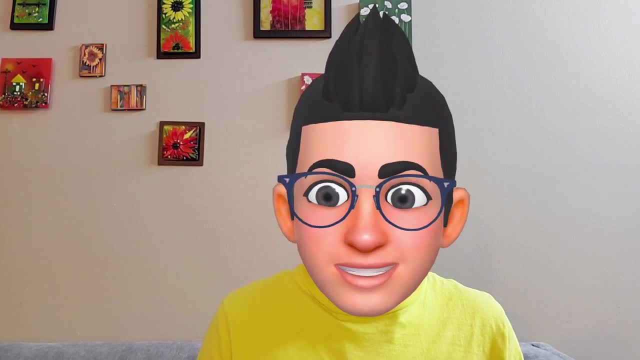 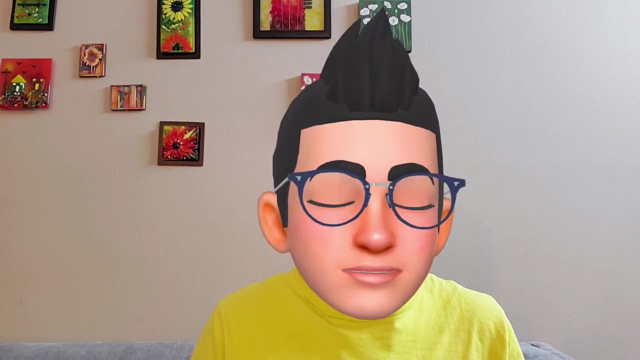 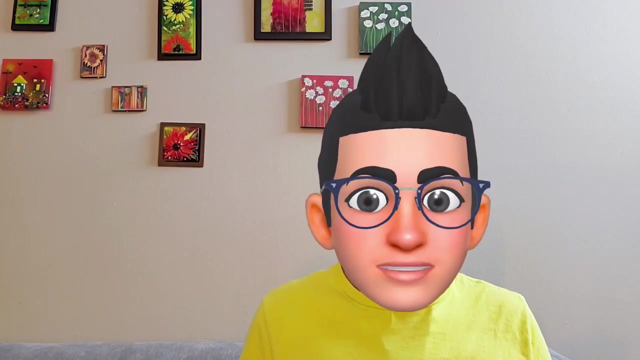 Now that you know C and you know electronic, it's time to move on and build and program a robot. A DIY do-it-yourself robot kit is probably the best tool if you want to get hands-on experience with robotics in short amount of time, with minimum cost. I did some research and I read about a few. 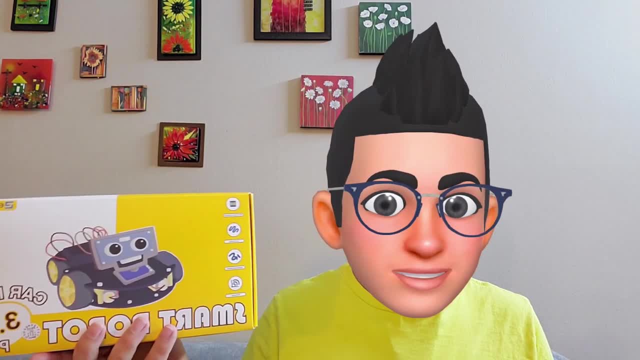 DIY robot kits. and finally, I found this robot kit by Elegoo- Did I say it right? Elegoo- which is well-priced, and it's a robot kit that you can use to build and program a robot. It's a robot kit that. 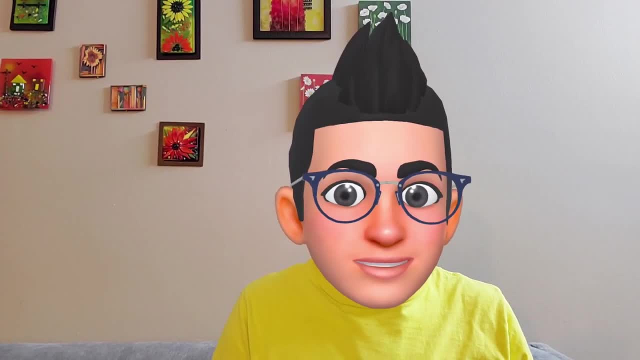 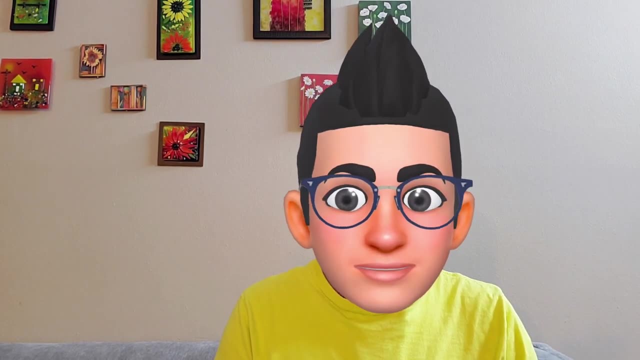 is highly rated on Amazon. I contacted them and then they sent me a sample to test out and review. They also offered you guys a promo code that you can use to get some additional discounts Again. the link and the promo code will be both down in the description section. 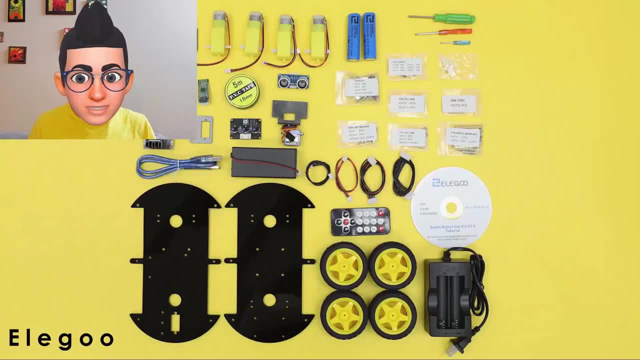 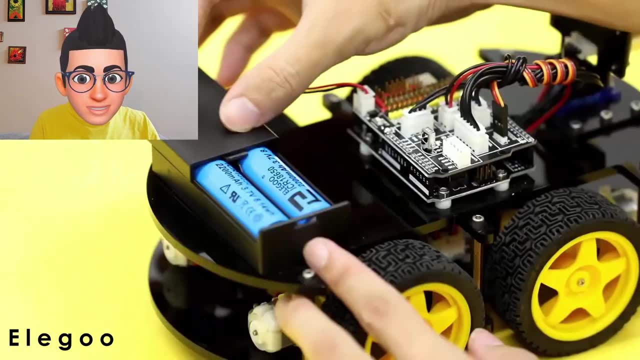 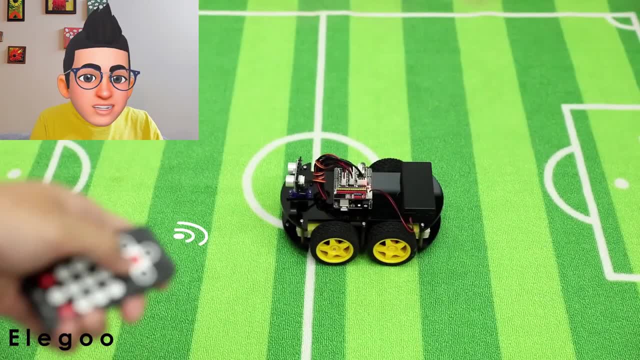 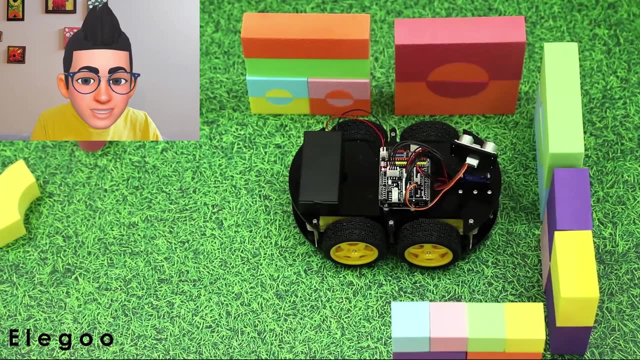 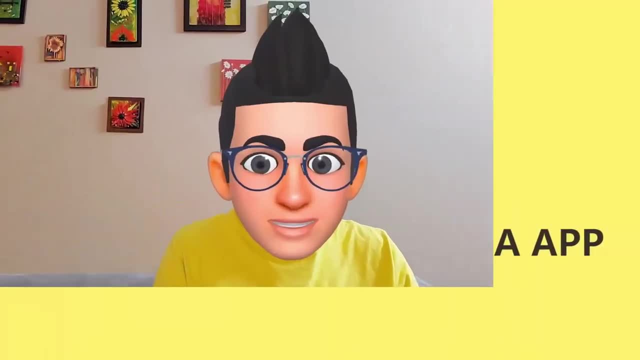 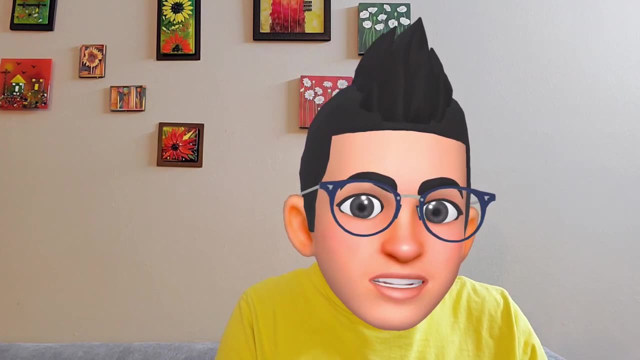 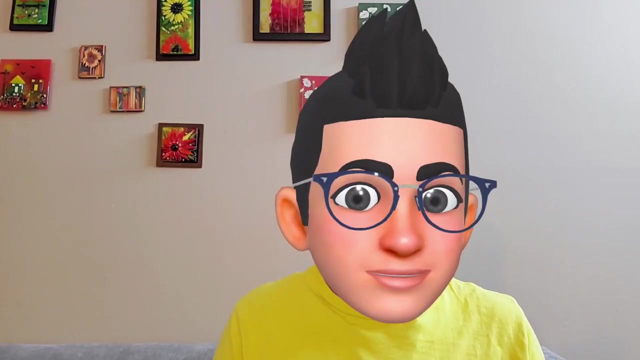 So that's the second reason: this is a great kit to learn robotics. And the third reason is this kit comes with 7 easy-to-follow lessons In. English is not your first language, Don't worry, because these lessons comes in French, Italian and Dutch. Okay, we talked about the good things. 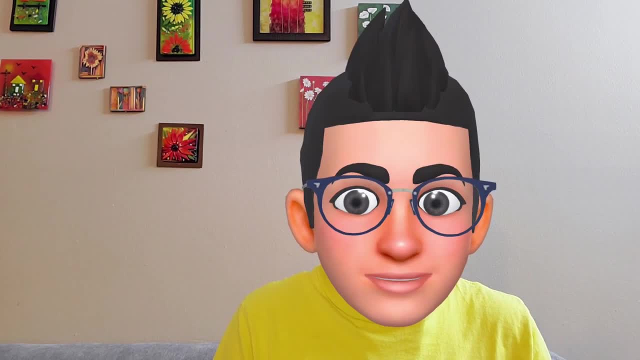 about this robot kit. they are quite hammering, but if you are still considering this, I would highly recommend you to start using it And once you begin to learn the水 community, the are some points that you need to keep in mind when you try to assemble this kit together. 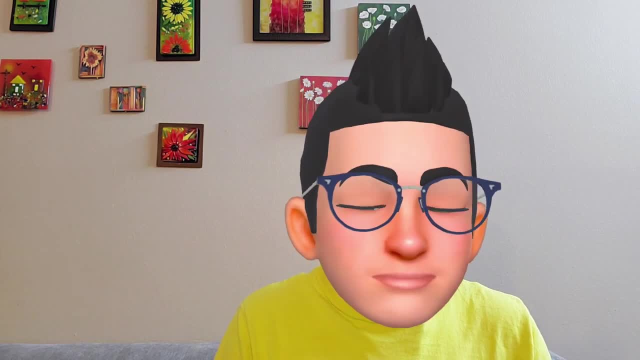 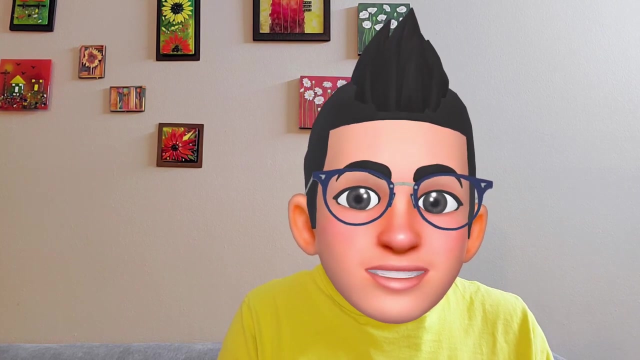 first, the assembly instructions is clear but it's not too detailed. maybe they did it on purpose to challenge you a little bit, so please be patient when you try to follow the instructions to to put this kit together. and second, the app to control the robot is easy to use but may not work. 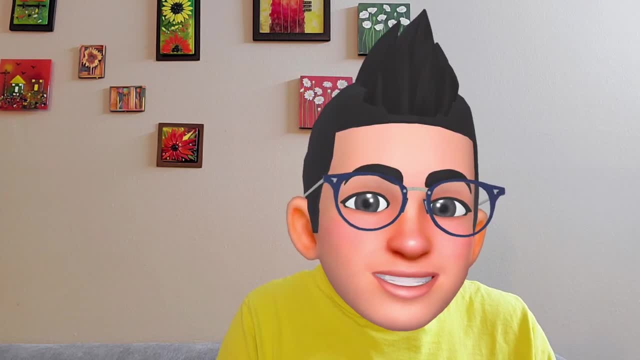 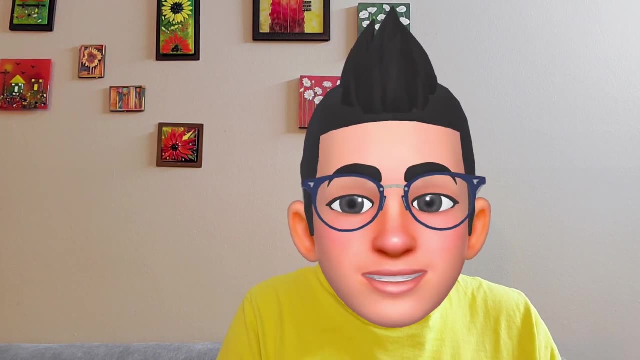 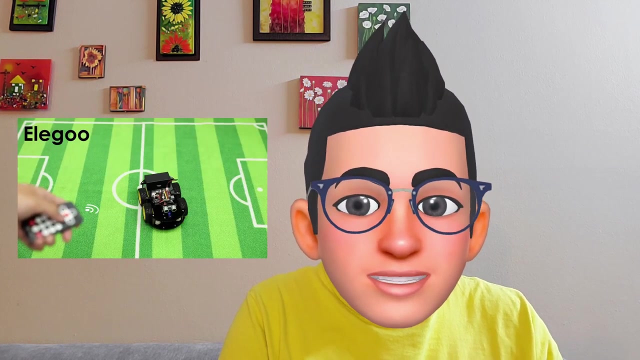 right out of the box. however, you do not really need the app. in my opinion, the app is designed mainly for kids who just want to have some fun with the robot. and then eventually, the robot comes pre-loaded with the default program that is controlled via the remote controller. it may or 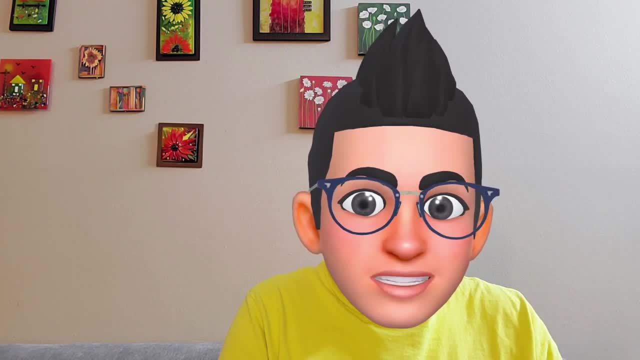 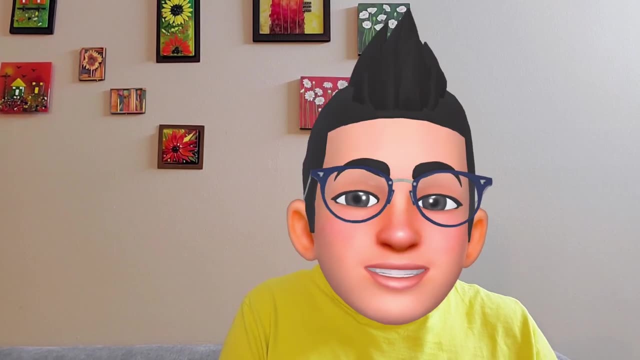 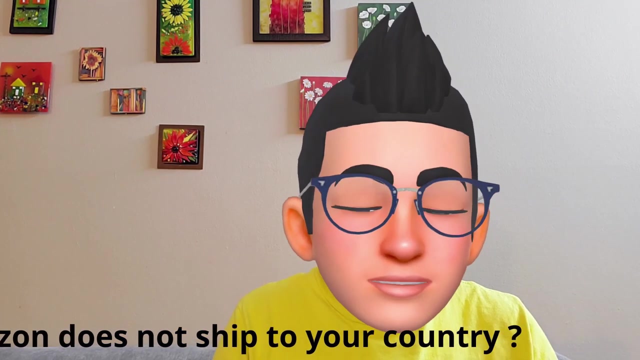 may not work properly. so it's better to follow the lessons in the tutorial folder and load the program to get it to work properly. please keep in mind that these lessons have not been designed to. i mean have been designed to get you started, but they may not be detailed enough for you to. 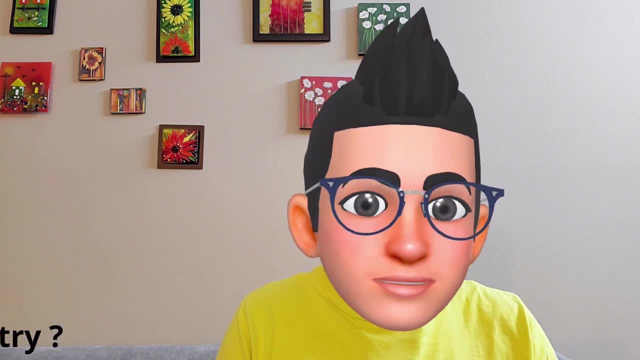 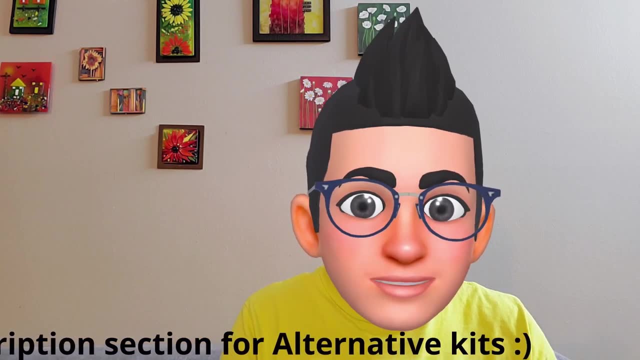 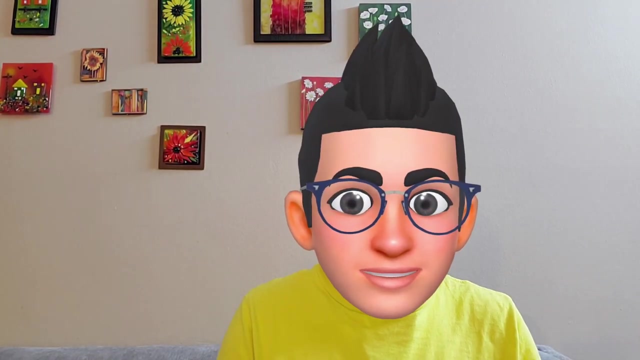 understand what's going on under the hood. so i'll put some references and additional resources down in the description section that you can watch and follow to get a better understanding of the electronics and how the program works and everything all right. so now let's summarize all three steps. step number one: learn c as the programming language you need to. 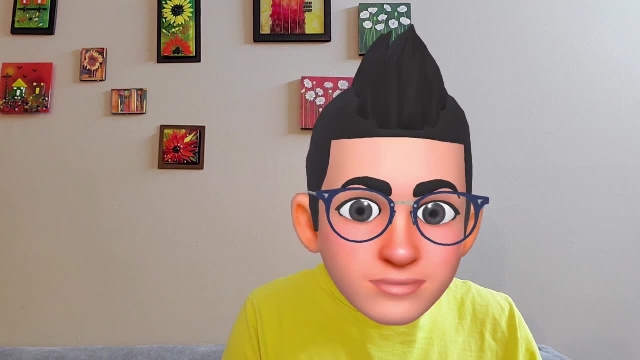 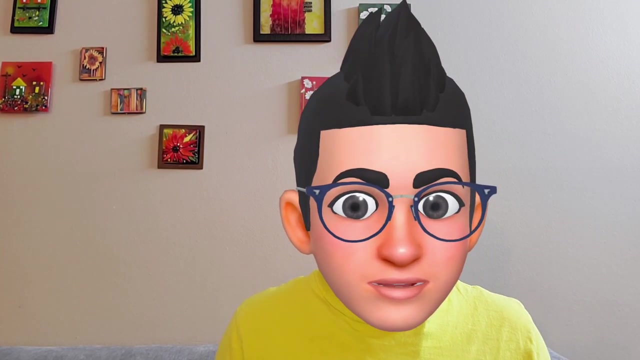 learn for robotics. step number two: buy an arduino kit and learn electronics using the arduino kit. step number three: buy a diy robot kit and learn how to build and program a robot. and please keep in mind that the goal of this video was to get you started with robotics, so if you want to become an expert, 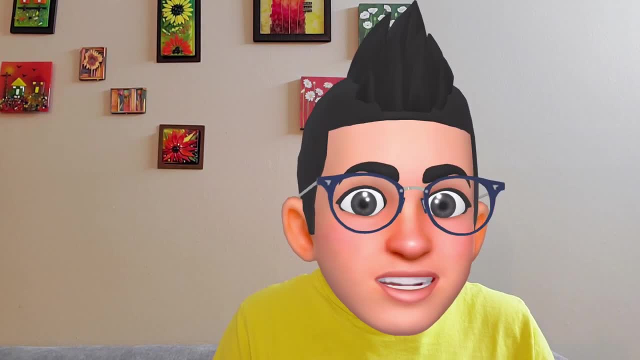 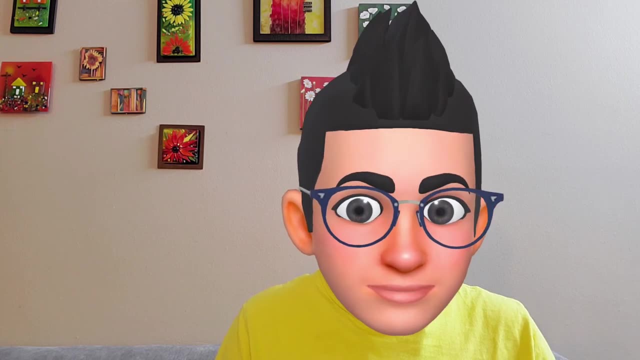 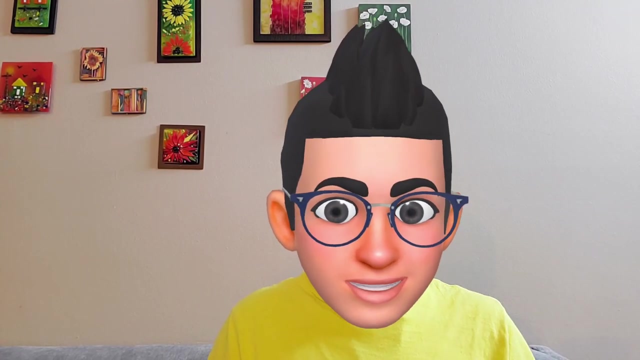 in robotics or if you want to become a robotics engineer. there's definitely more to it than this video, but we are planning to create more videos for people who want to go from a beginner to a robotics engineer or an ai engineer, so thank you very much for watching this video.